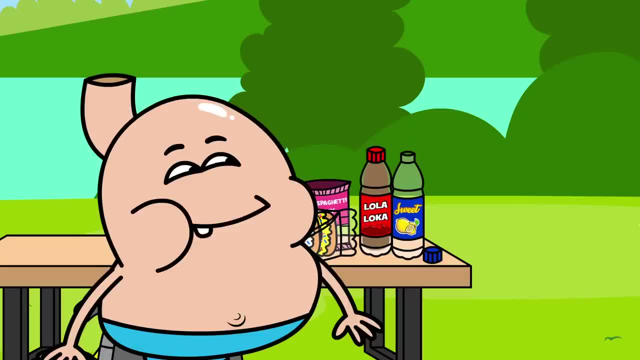 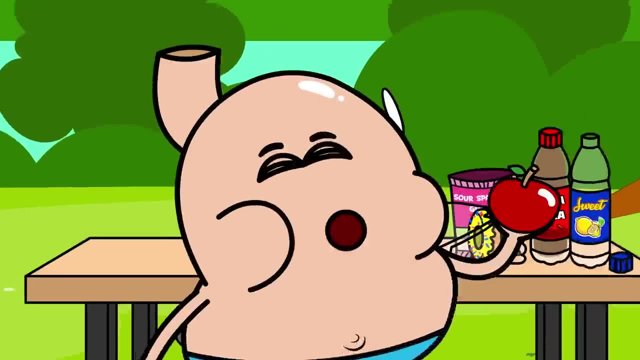 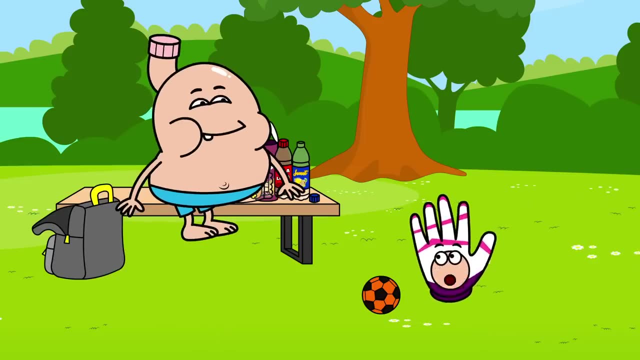 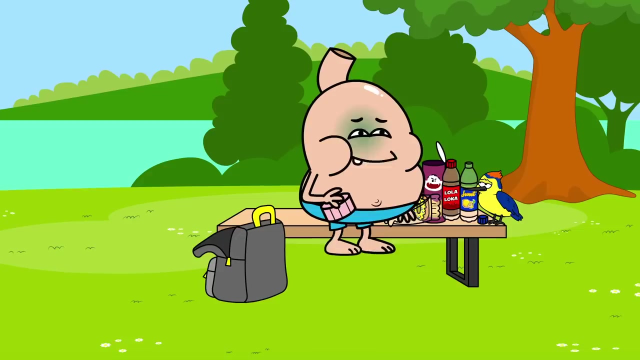 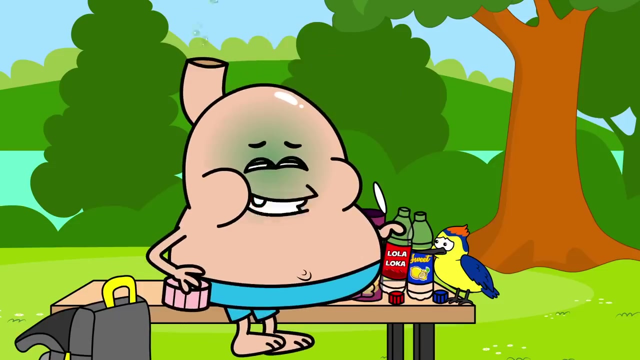 Hello, Lulu, Tweet. Oh, oh, oh, oh, Tweet. Ha, ha, ha, ha, no, Hey, Tommy play ball now. Oh, oh, oh, no, Oh, Hmm, Oh, I feel sick. Twiddle dee, dee, twiddle dee, dee. 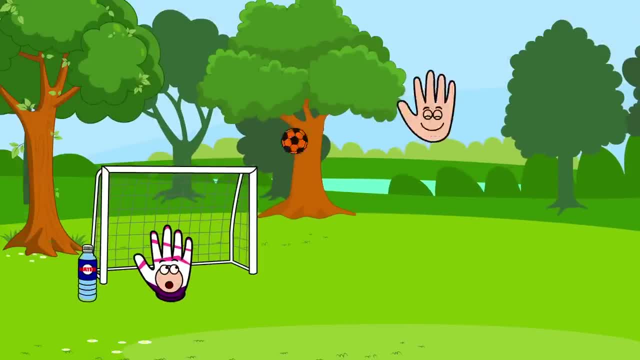 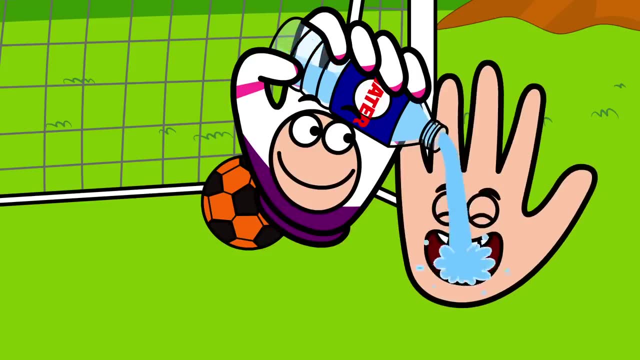 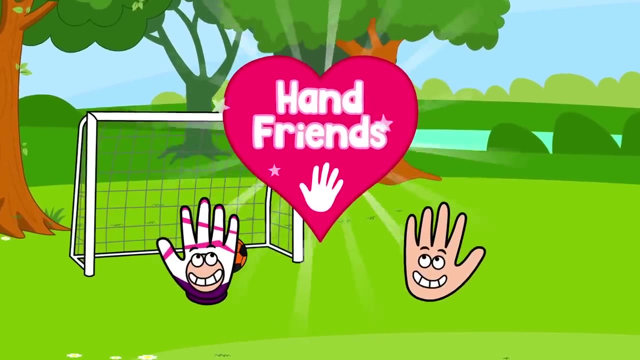 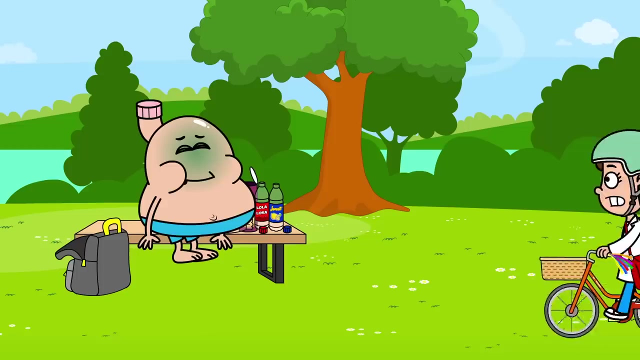 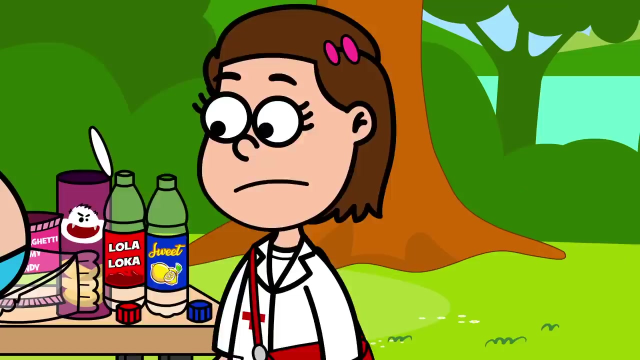 Twiddle, dee, dee, dee, Yep, yep, bam, Ah, handball, Hand. friends, Tommy, I come to save you. Oh, Tommy, you look sick. I am very, very sick. So much fat, sugar and salt. 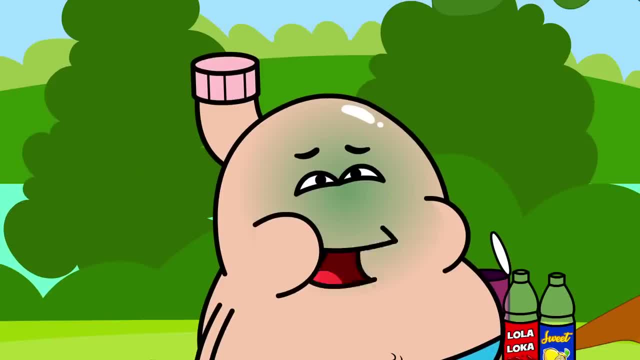 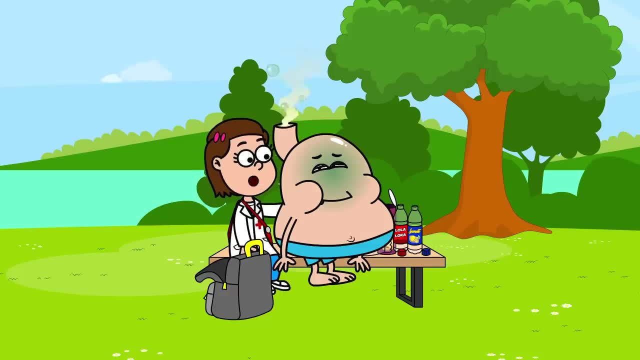 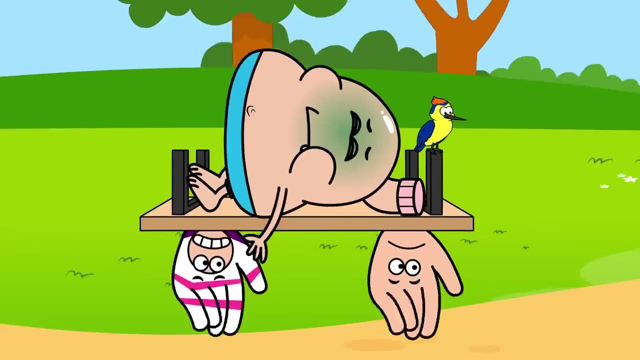 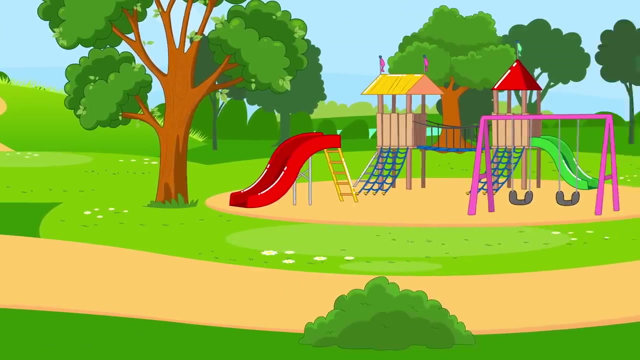 Not good for Tommy. Yummy, Tommy, where is my mommy? I take you to my hospital, But how Mmm, sweet and salty Mmm, so yummy. But too much is not good for you, Tommy. The best that you can feel. 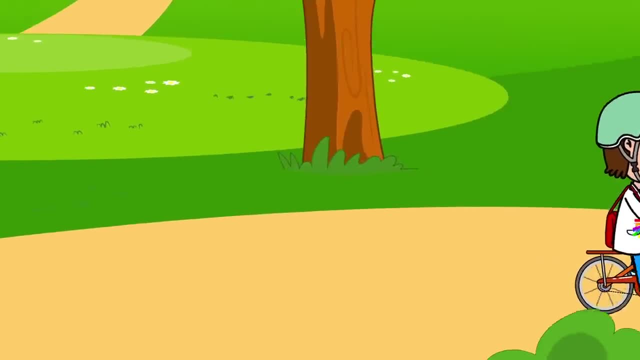 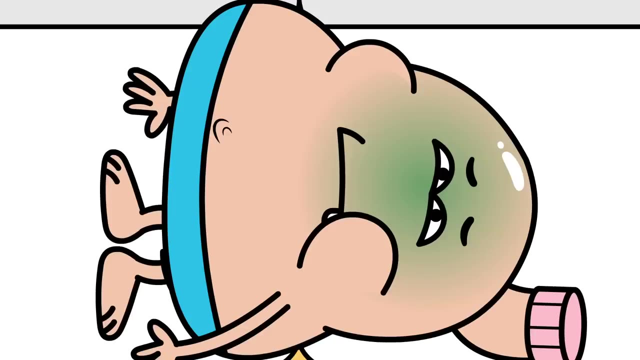 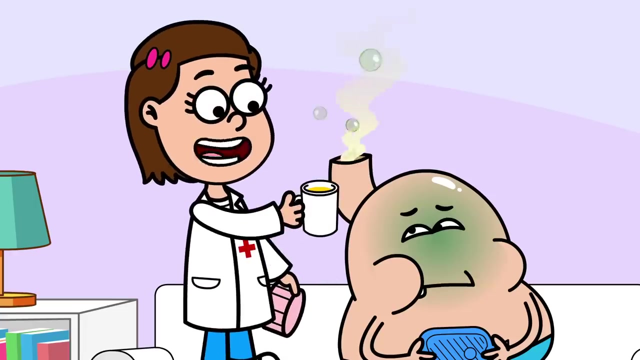 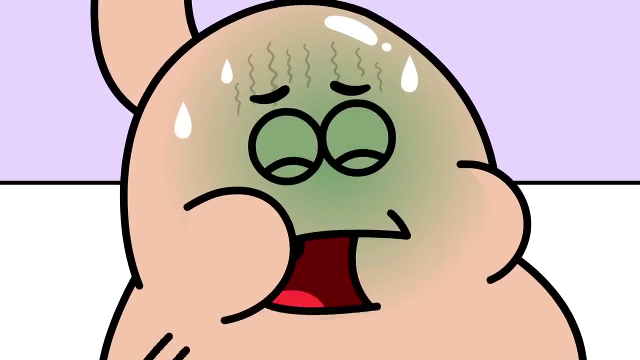 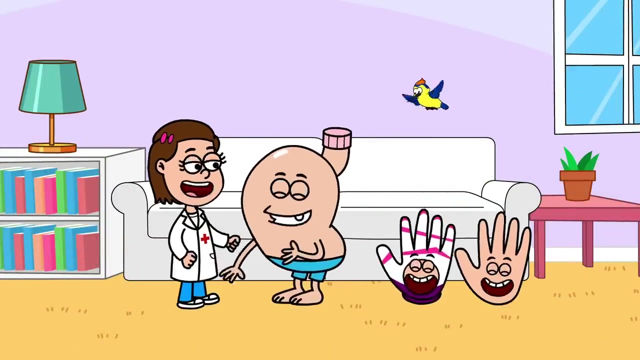 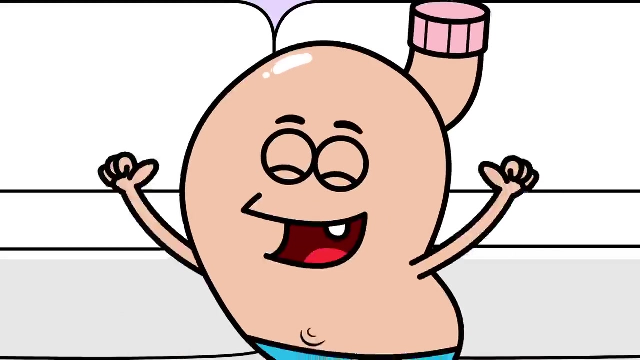 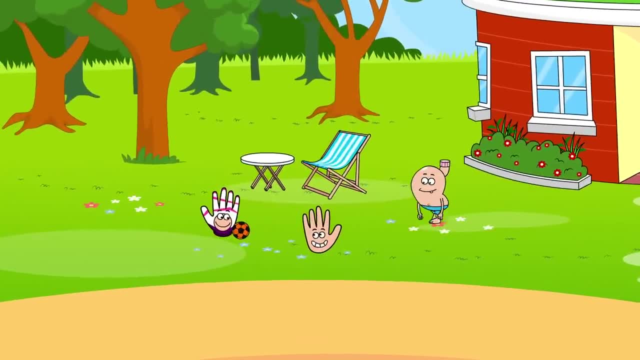 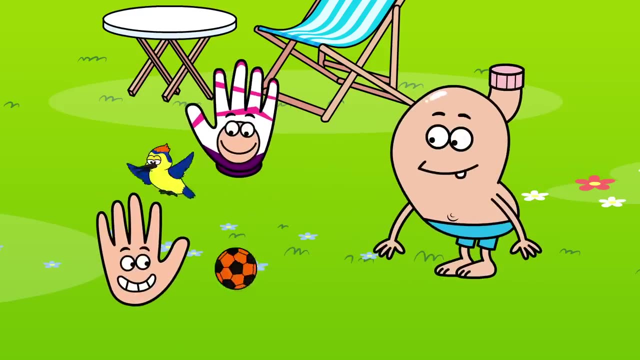 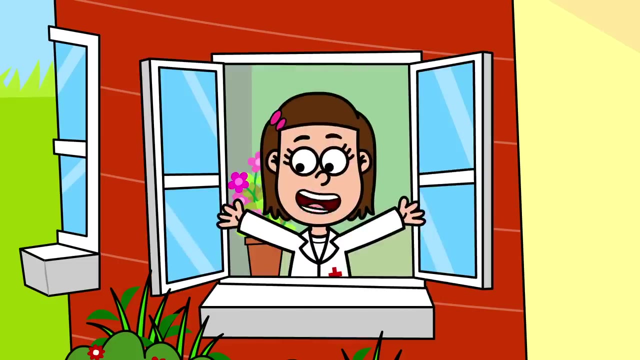 Mmm, Mmm, Mmm. Hey, Tommy, play ball. Yes, Yay, Sweet and salty Twiddle dee, Mmm. so yummy Twiddle dee, But too much is not good for you. Tommy Time for a happy Tommy meal.